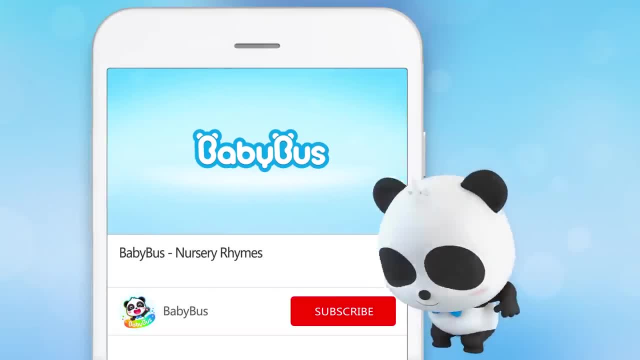 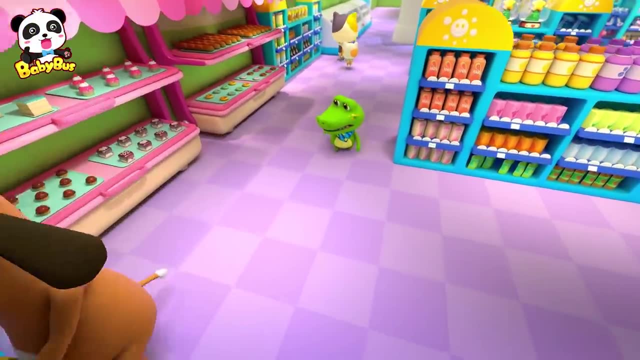 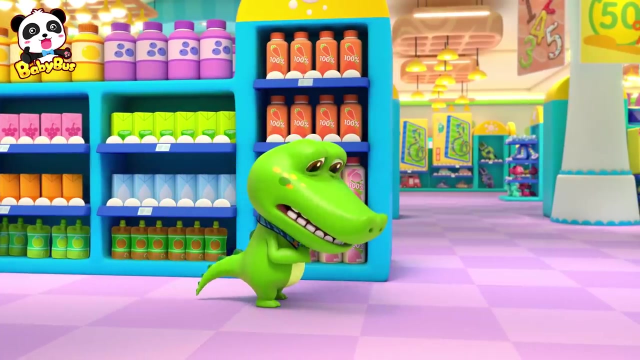 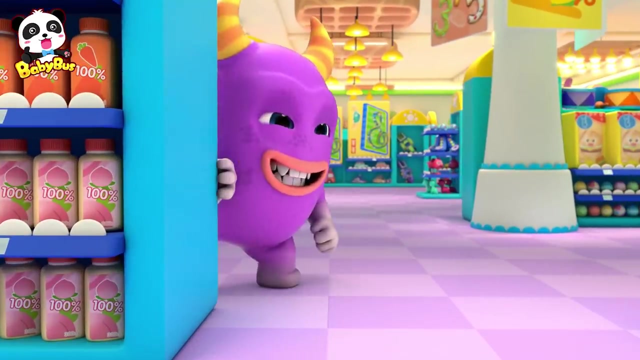 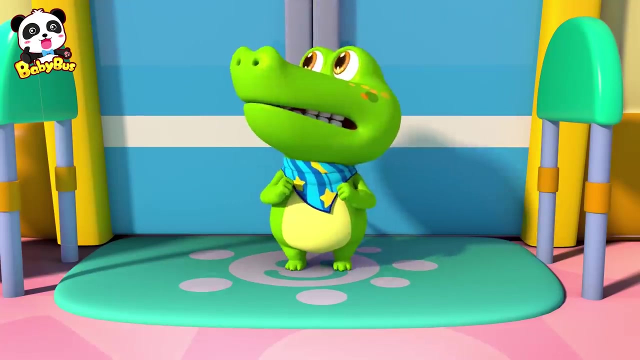 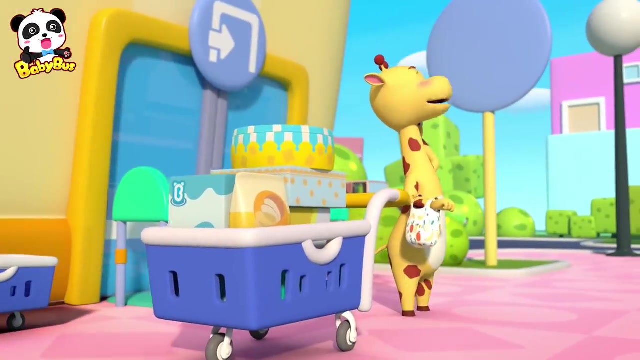 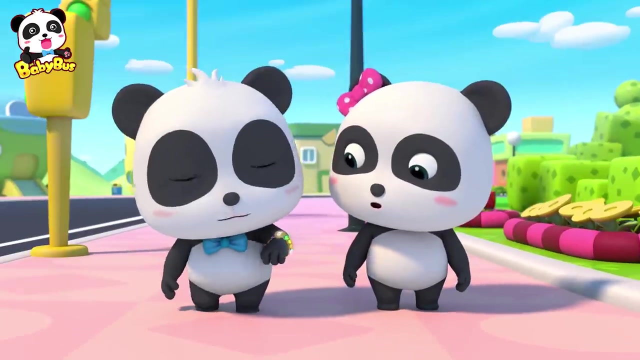 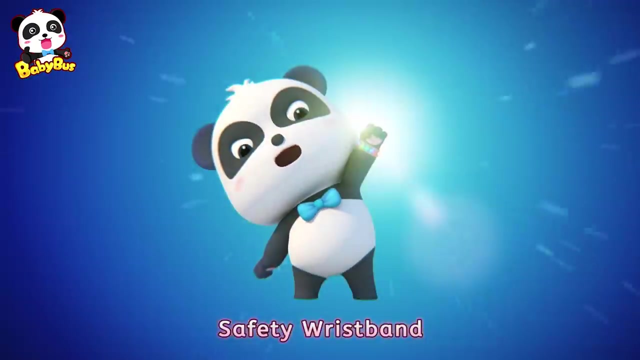 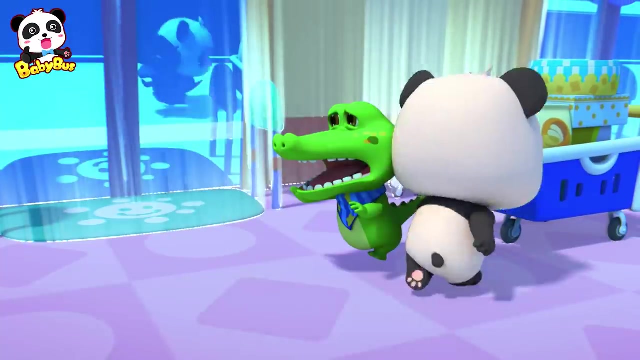 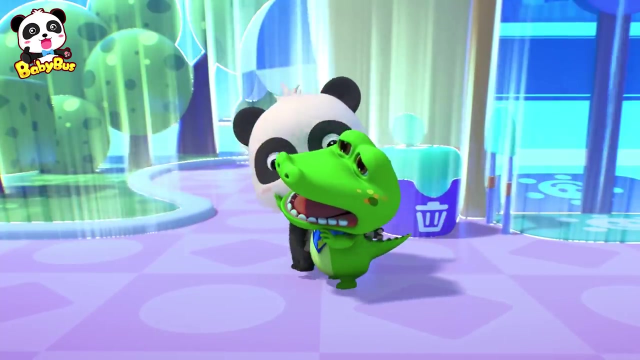 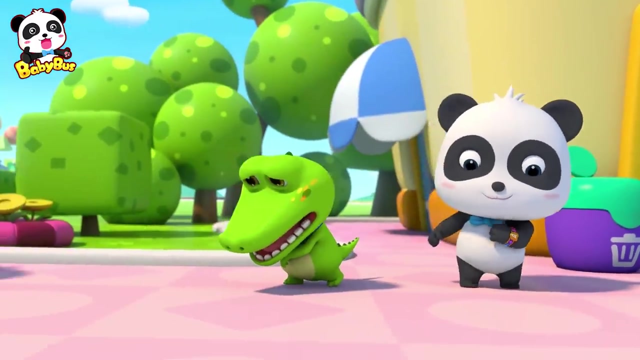 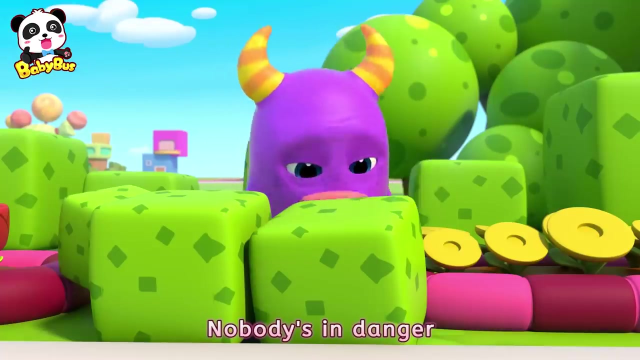 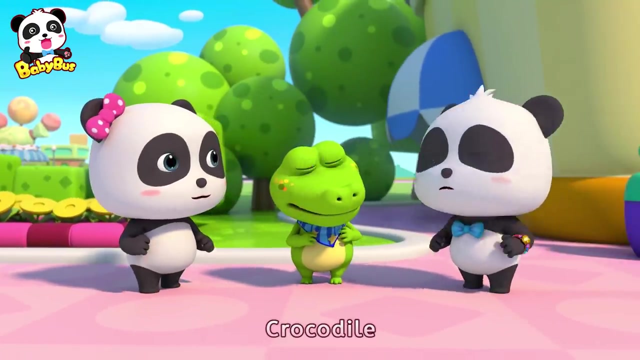 Baby Bus. Click here to subscribe. Mommy, mommy, where are you? Danger is coming. Oh Yeah, I know. Safety wristband. spin, spin, spin. Hey, Nobody's in danger. I don't like it. Crocodile, why are you here all by yourself? Where's your mom and dad? I? 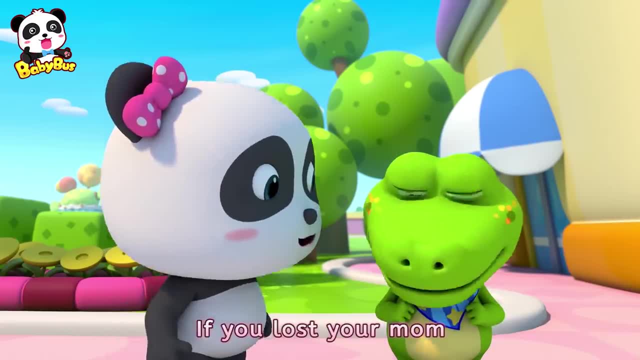 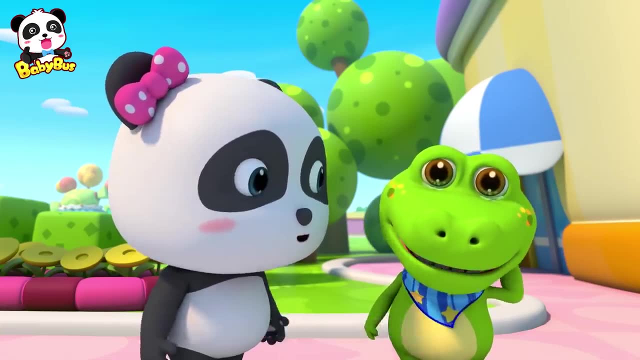 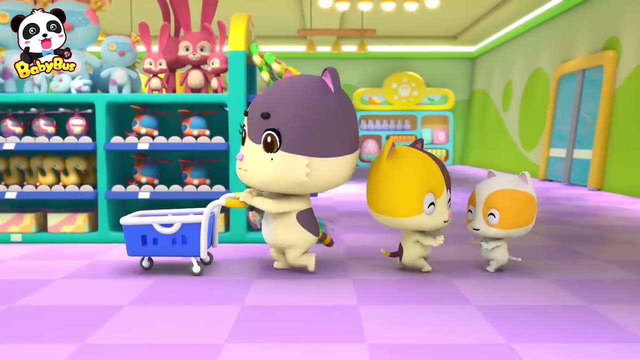 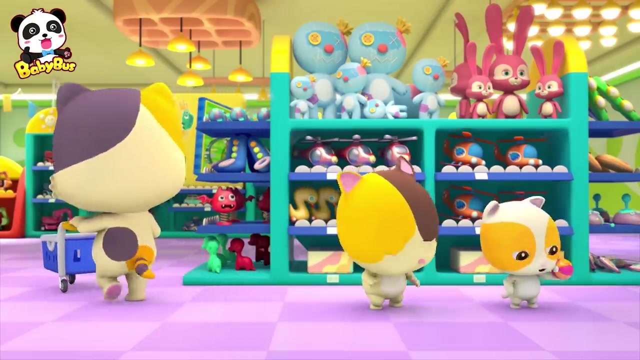 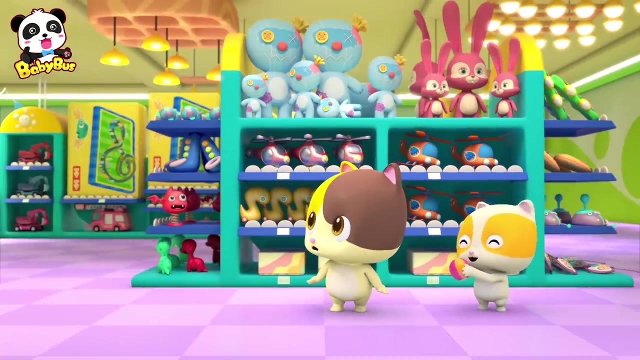 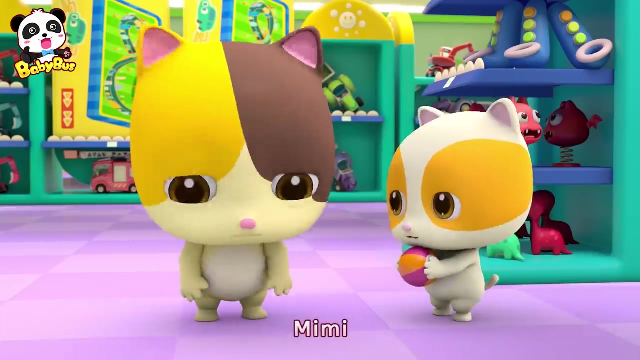 Can't find my mom. If you lost your mom, you shouldn't be running around, Then why should I do? let's take a look. Stay close to mommy. Oh, Mommy, look, Mommy, Mommy, Oh no, Mommy, mommy, Oh no, Mimi, where's mommy? 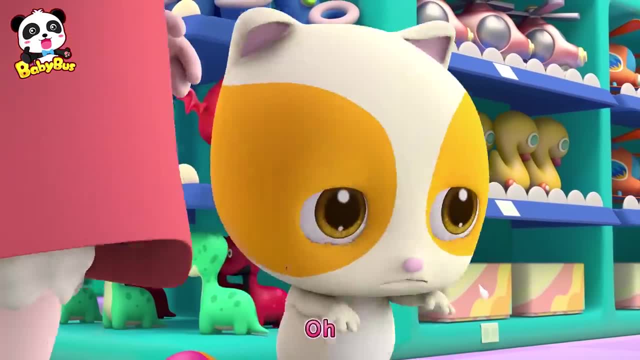 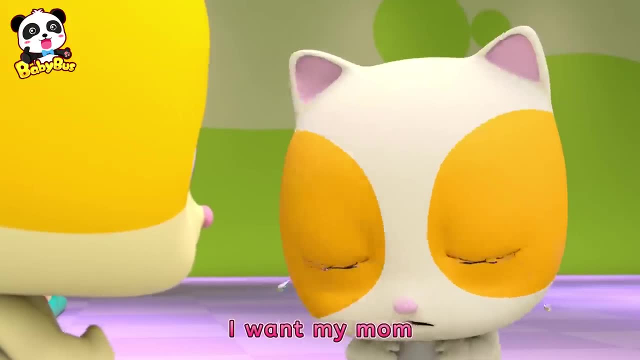 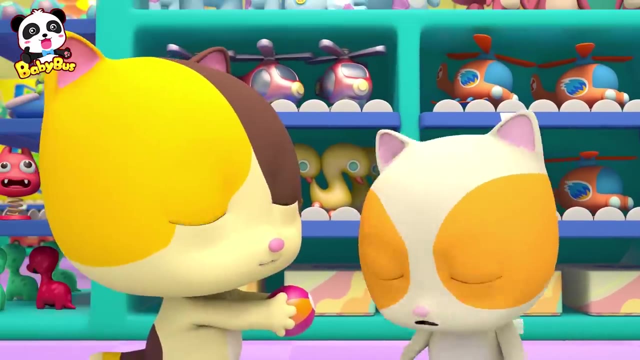 We're lost. We are lost, Oh, we are lost. I'm so scared, boo hoo, hoo. Oh no, I want my mom. Don't worry, don't cry, Let's wait for mommy here. Don't worry, don't worry, Let's wait for mommy here. 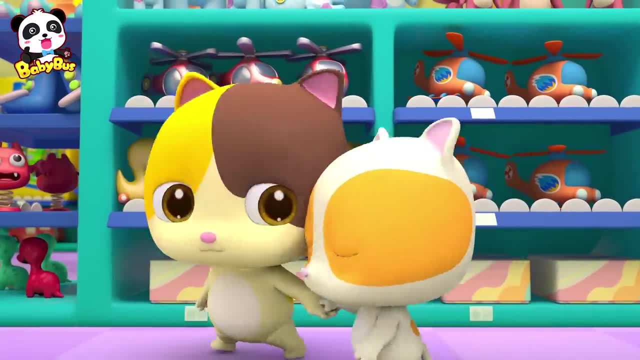 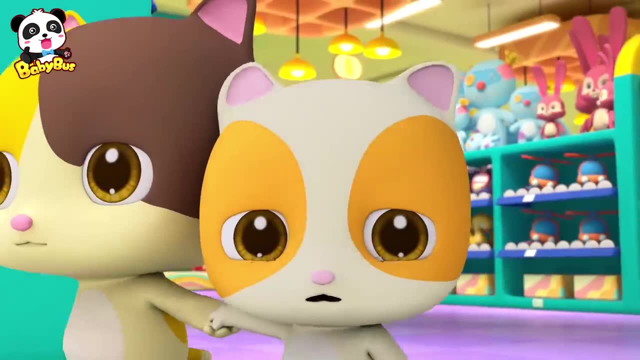 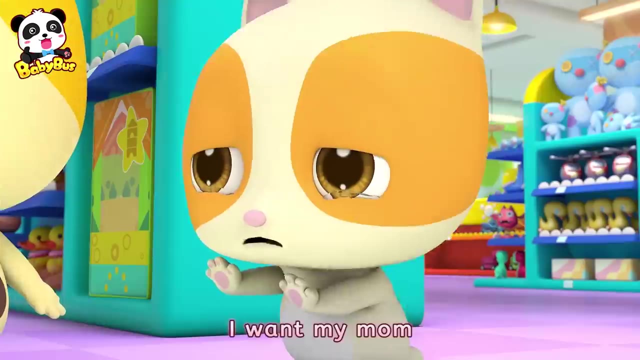 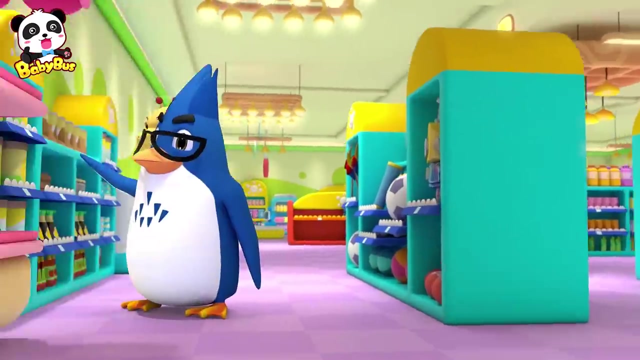 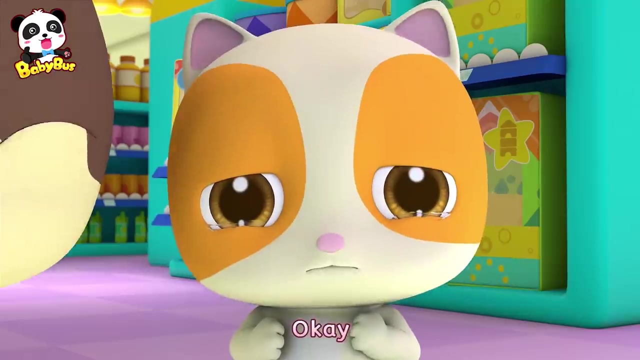 Mommy's not coming. Who can help us? We are lost. we are lost. I'm so scared. Oh no, oh no, I want my mom. Don't worry, don't cry. Find someone in uniform Over there. over there, She will help us. Okay, let's ask her for help. 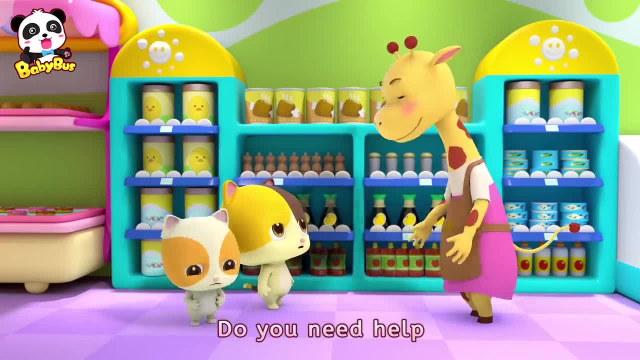 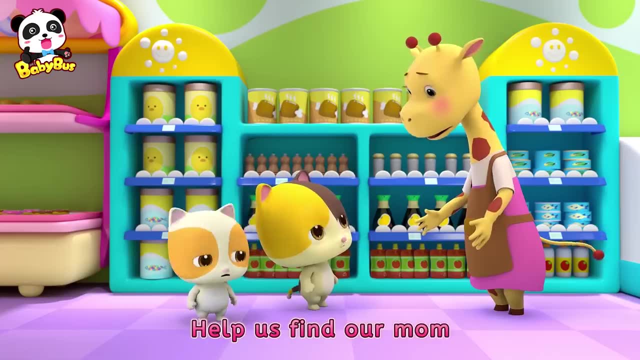 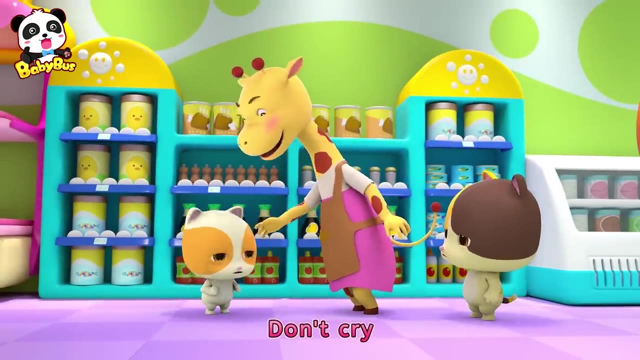 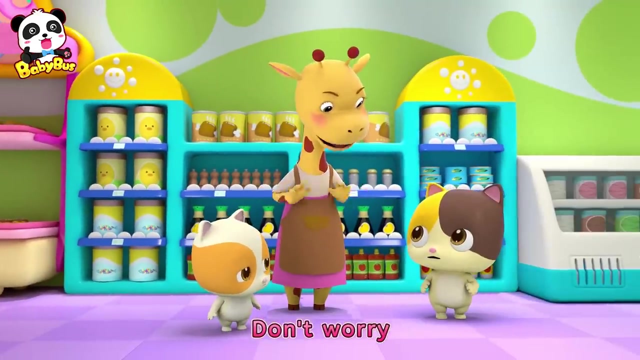 Kids, do you need help? We are lost. oh, we are lost. Help us find our mom. Oh no, oh no, I want my mom. Don't worry, don't cry, I'll help you find your mom, Don't worry, don't worry, Follow me, little kids. 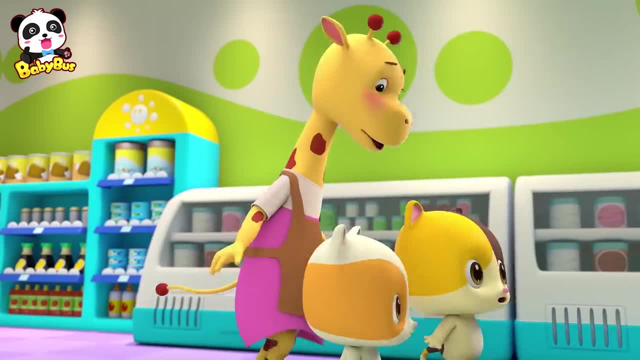 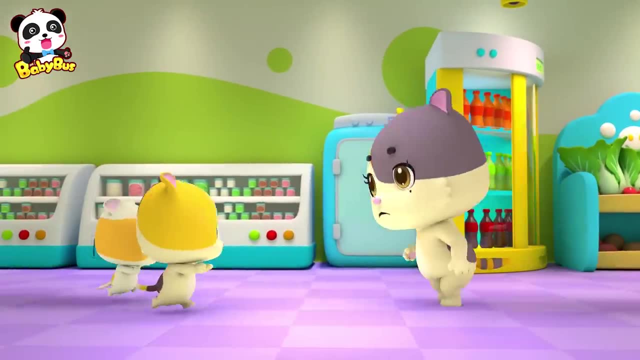 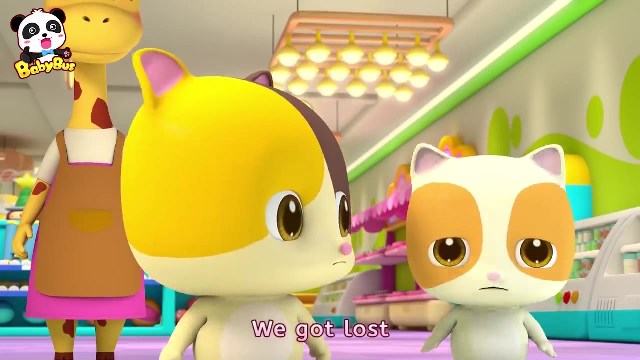 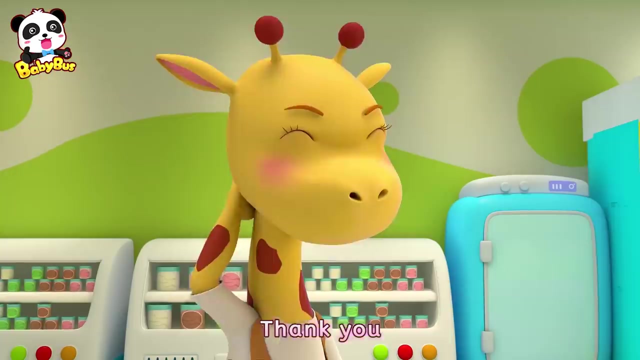 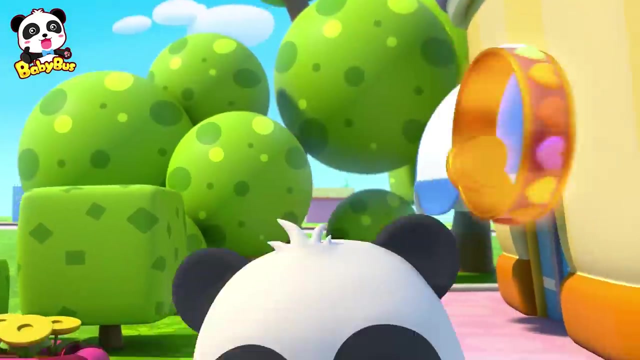 Okay, thank you, It's mommy, Mommy, mommy, mommy, Mimi, Timmy, Where have you been? We got lost. yeah, This lady helped us. Thank you, You're welcome. Always stay close to your mom. Okay, Ha ha, ha, Got it. 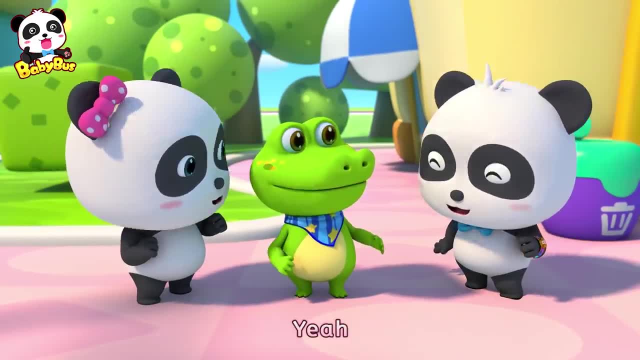 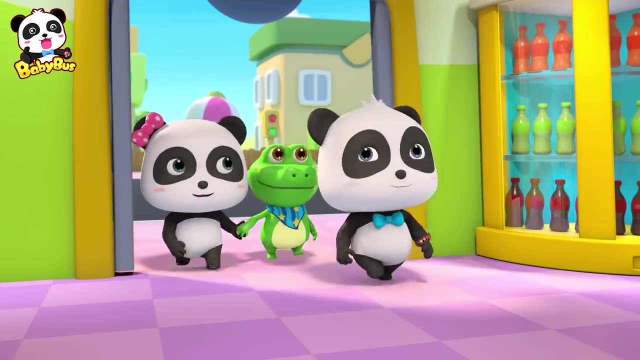 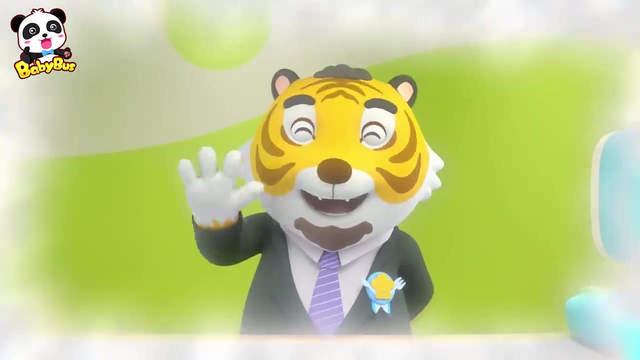 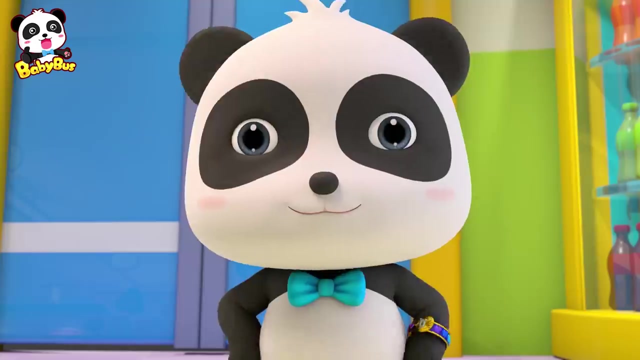 I'll go back to the mart and wait for my mom there. Yeah, If you still can't find your mom, Then we should go to customer service and ask for help. Hi Ha, ha ha. There are a few things to remember if you're lost. Let's take a look. 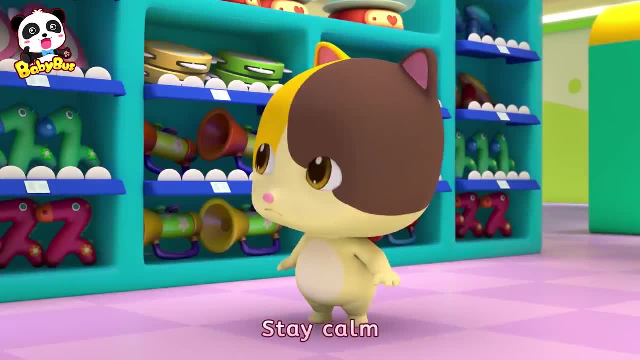 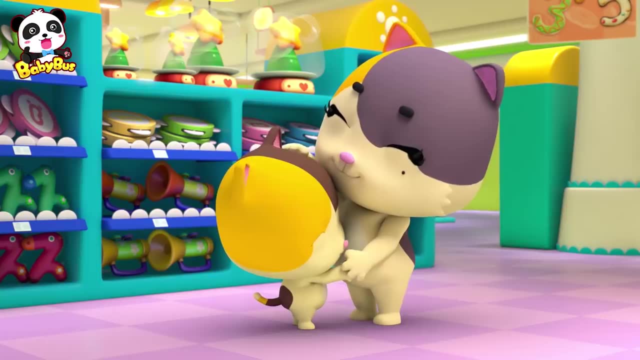 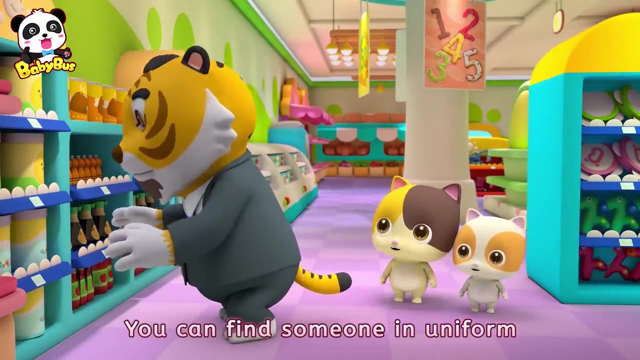 First, stay calm, stay where you are And call out your parents' name. Oh ha ha ha. Remember your mom and dad's phone numbers. You can find someone in uniform And ask them to help call your mom and dad. Oh ha ha ha. 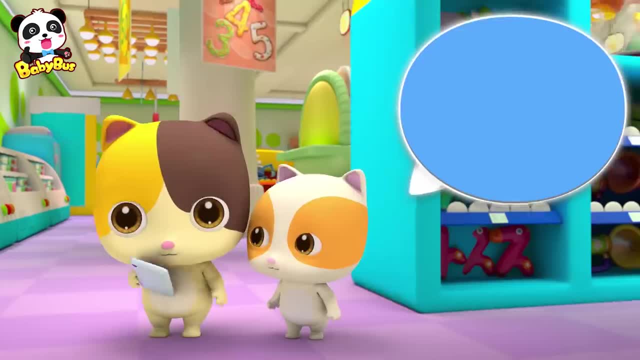 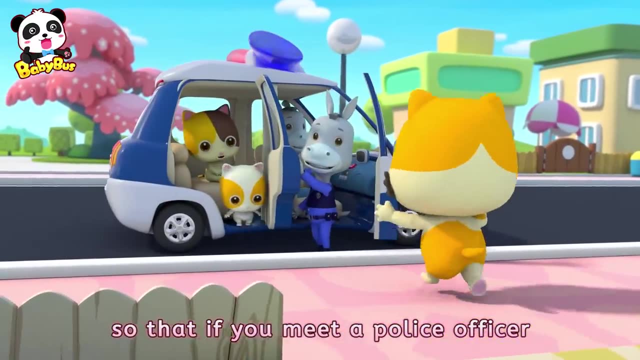 Hello mom, Mimi, Also, remember your home address So that if you meet a police officer, You can ask him to take you home. Ha ha, ha, ha, Ha ha ha. Hey, Daddy, Ha ha, ha ha.